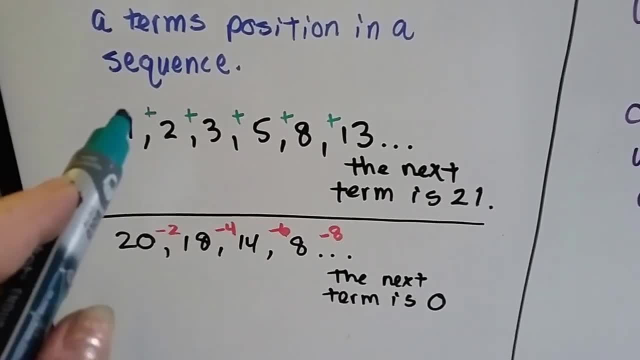 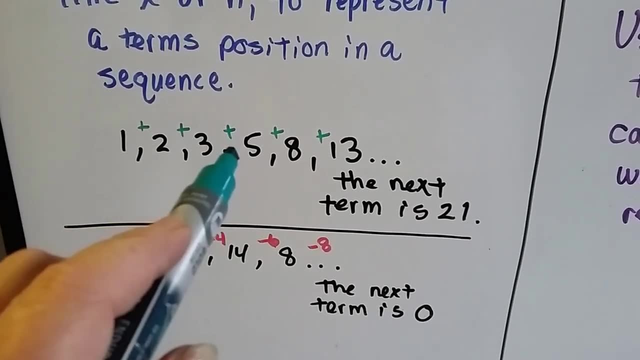 the first one in the second one we're doing. In the first one, when we added the one plus the two, we got three. and we added the two and the three, we got five. and when we added this one, we got five. And this one, the three and the five, we got eight. Eight and five is thirteen. 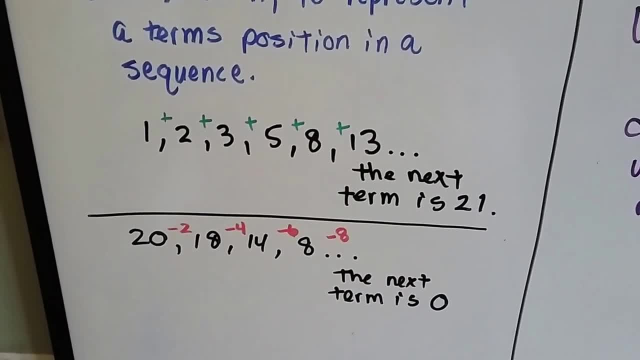 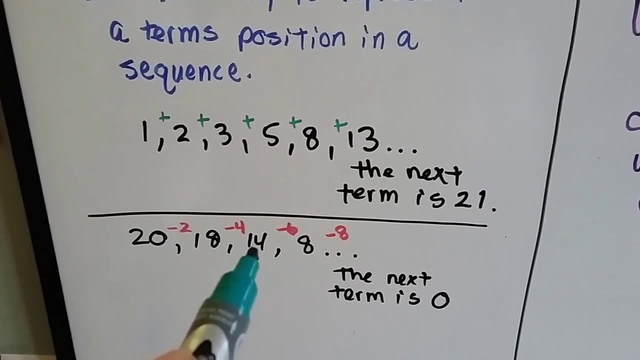 Thirteen and eight is. the next one would be 21.. In the other one that was decreasing, it went 20, then 18, so it went down by two. From the 18 it went to 14, it went down by four. From the 14 it went to eight. that's down by six. See what's. 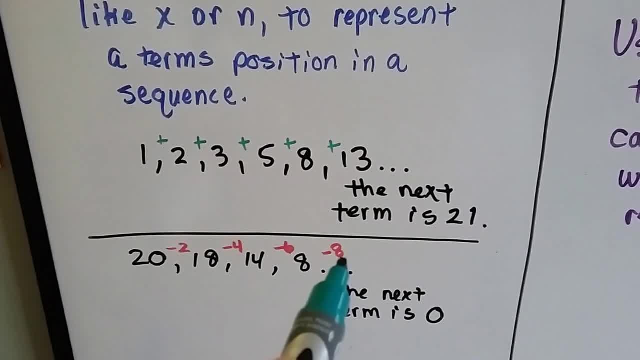 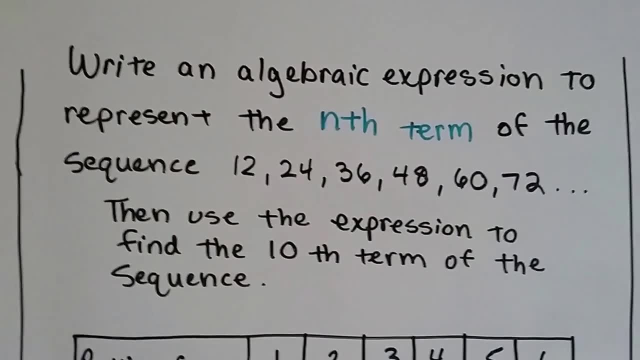 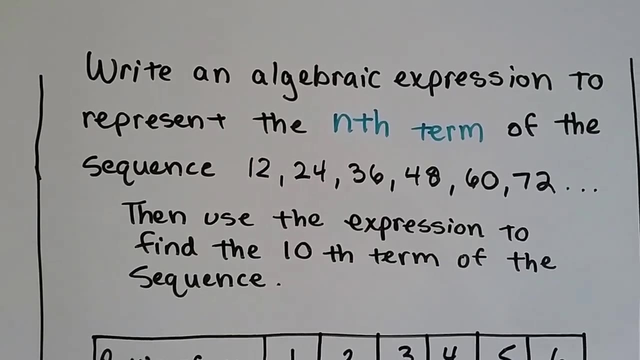 happening. Skip counting and subtracting, So the next one is going to be negative eight, it's going to be a zero. See, So we can write an algebraic expression to represent the nth term of a sequence. So if we did it for 12,, 24,, 36,, 48,, 60,, 72, we could then use: 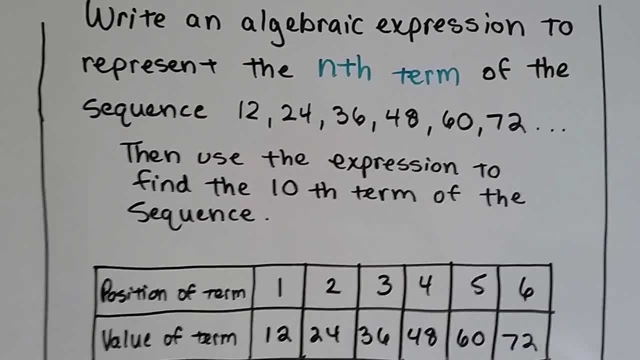 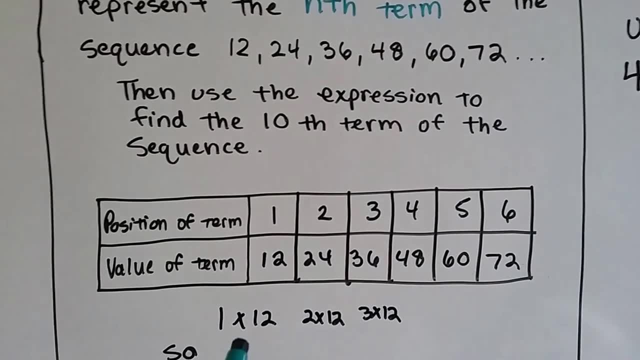 the expression to find the 10th term or the 11th or 12th of the sequence. Make a little chart. We write the position of the term and the value of the term. We can easily see that 1 times 12 is 12. 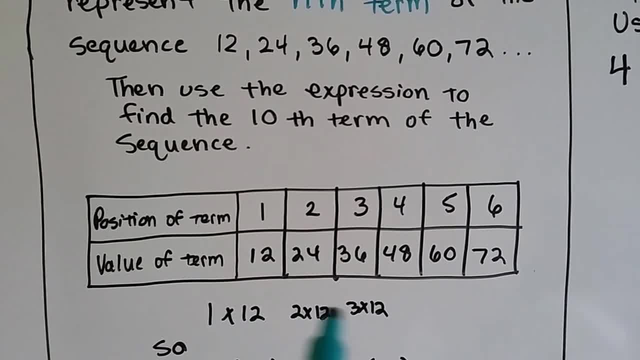 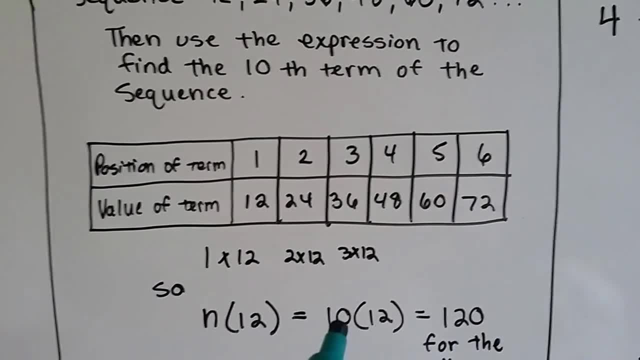 and 2 times 12 is 24, 3 times 12 is 36.. So we see that it's some number times 12.. So n times 12 is our expression that we can use to find the 10th term. 10 times 12 is 120.. That's the 10th term in. 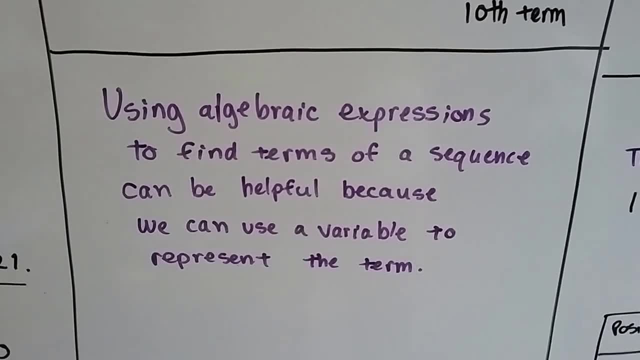 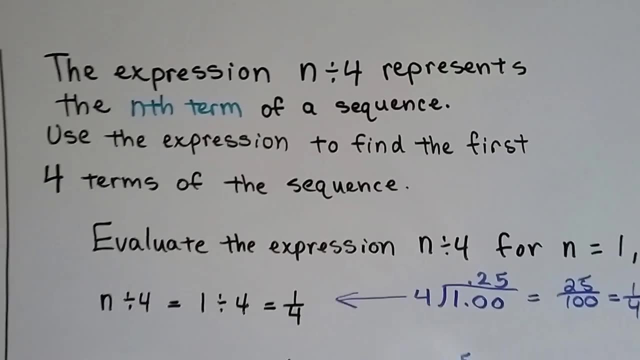 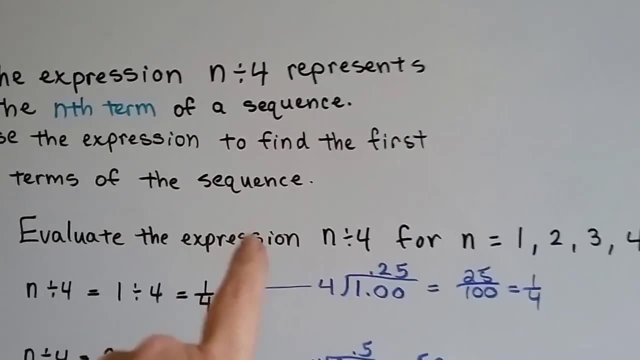 the sequence. So using algebraic expressions to find terms of a sequence can be helpful because we can use a variable to represent the term. The expression n divided by 4 represents the nth term of a sequence. Use the expression to find the first four terms of the sequence. So we 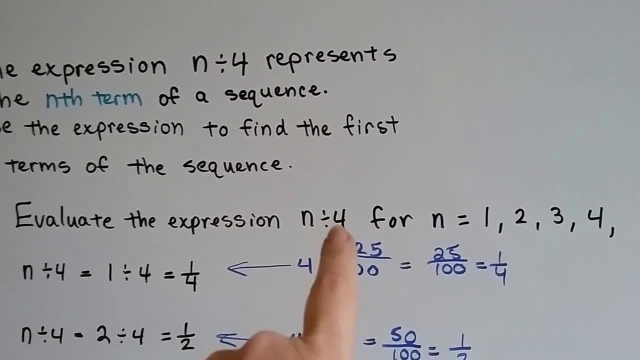 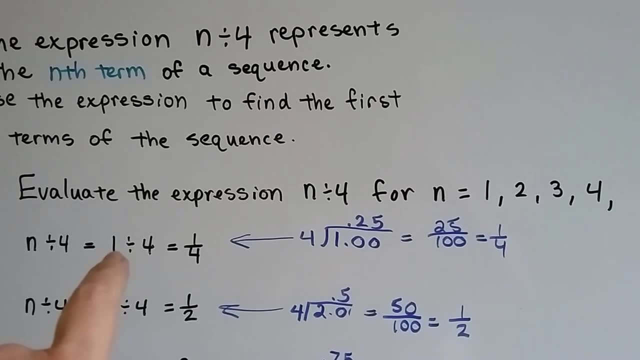 got 1,, 2,, 3,, 4.. Evaluate the expression n divided by 4.. If n equals 1,, 2,, 3, and 4.. So n divided by 4.. If n equals 1,, it would be 1 divided into 4.. 1 divided. 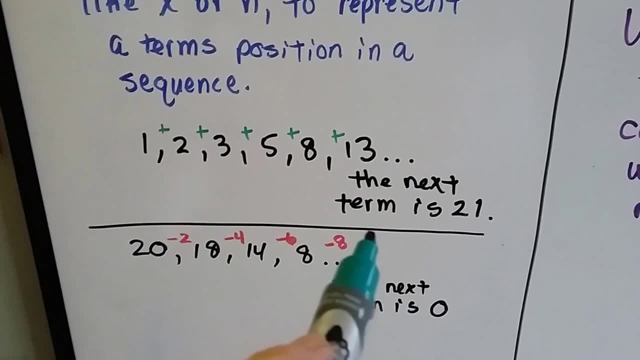 From the 14, it went to 8,. that's down by 6.. See what's happening. Skip counting and subtracting, so the next one's going to be negative 8.. It's going to be a 0, see. 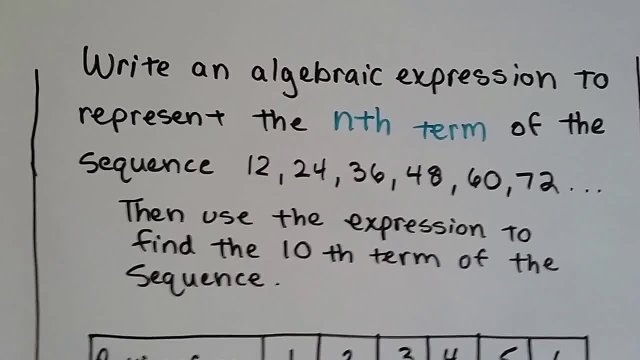 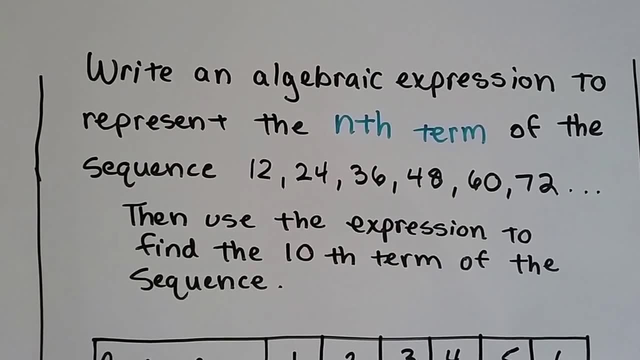 So we can write an algebraic expression to represent the nth term of a sequence. So if we did it for 12,, 24,, 36,, 48,, 60,, 72, we could then use the expression to find the. 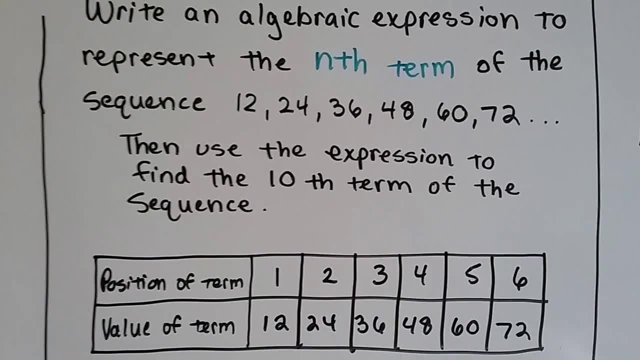 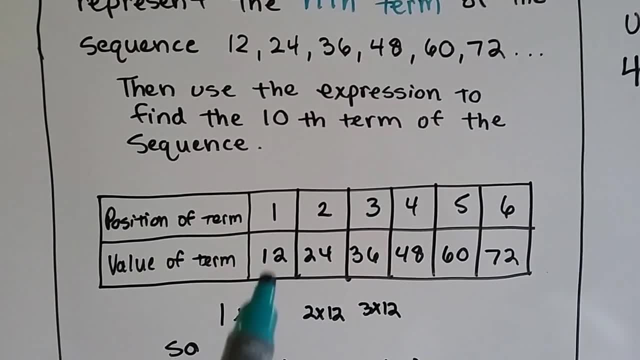 10th term or the 11th or 12th of the sequence. Make a little chart. we write the position of the term and then the value of the term. We can easily see that 1 times 12 is 12, and 2 times 12 is 24,. 3 times 12 is 36.. 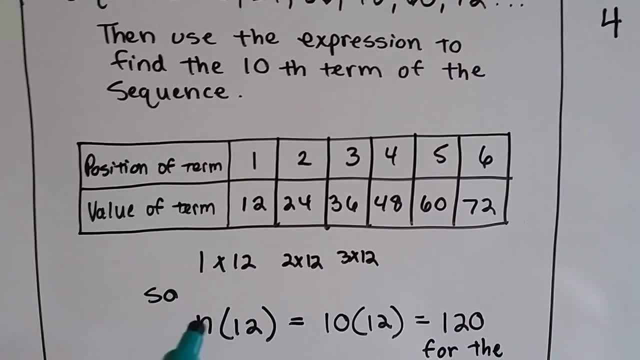 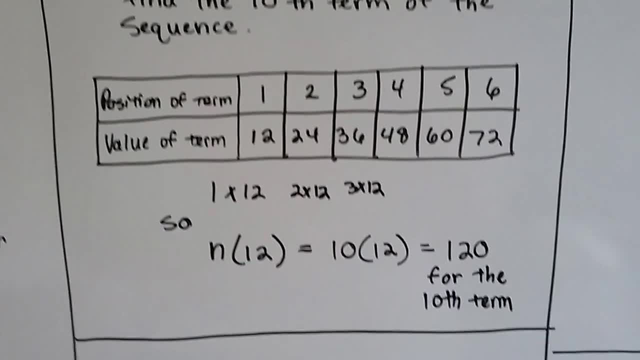 So we see that it's some negative. We can find the number times 12, so n times 12 is our expression that we can use to find the 10th term. 10 times 12 is 120.. That's the 10th term in the sequence. 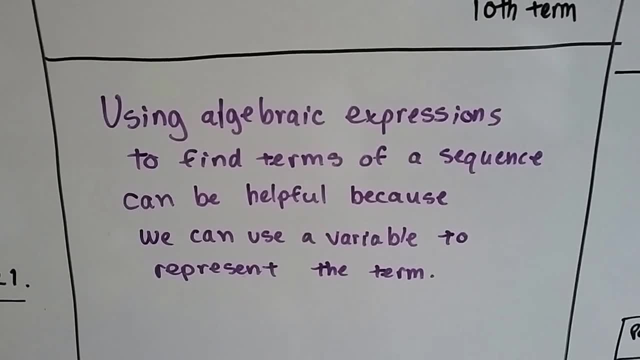 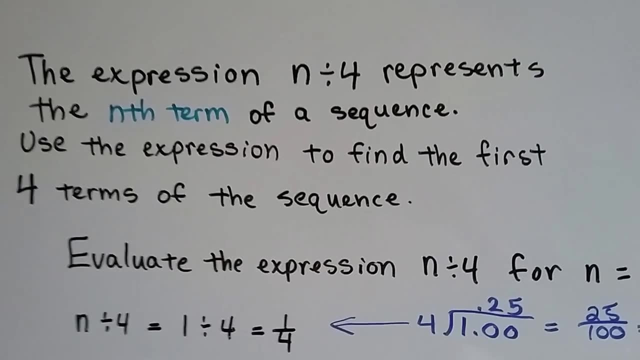 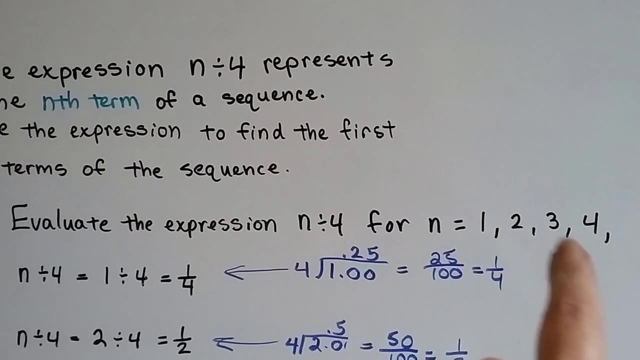 So using algebraic expressions to find terms of a sequence can be helpful because we can use a variable to represent the term. The expression n divided by 4 represents the nth term of a sequence. Use the expression to find the first four terms of the sequence. so we got 1,, 2,, 3,. 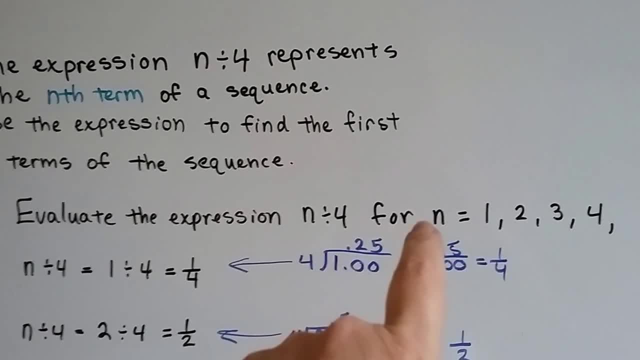 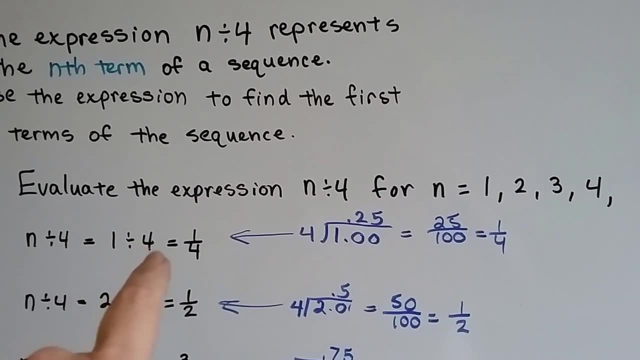 4. Evaluate the expression n divided by 4. if n equaled 1,, 2,, 3, and 4.. So n divided by 4,. if n equaled 1,, it would be 1 divided into 4.. 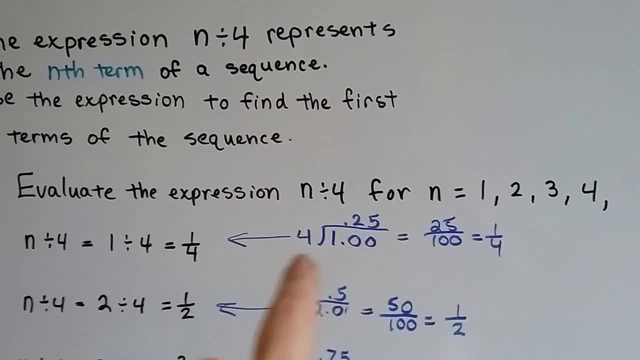 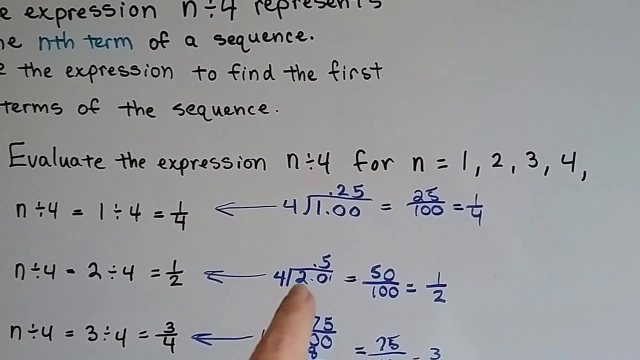 1 divided by 4 is 0.25, or 25 hundredths, or 1 fourth. If n divided by 4, if the n was a 2, see, then it would be 2 divided by 4, which is: 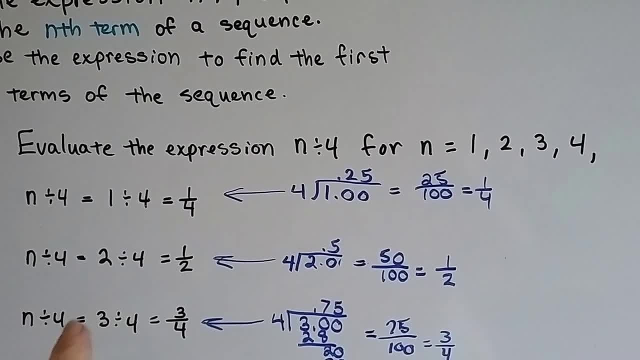 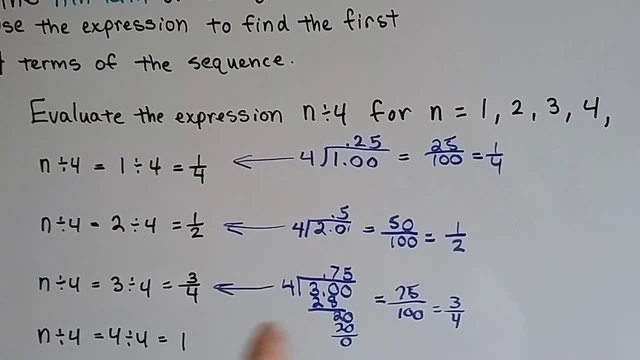 0.50, or 50 over 100, or a half. If it represented a 3,, it would be 3 divided by 4. And it would be 3 fourths, because 0.75 is 75 hundredths or 3 fourths. 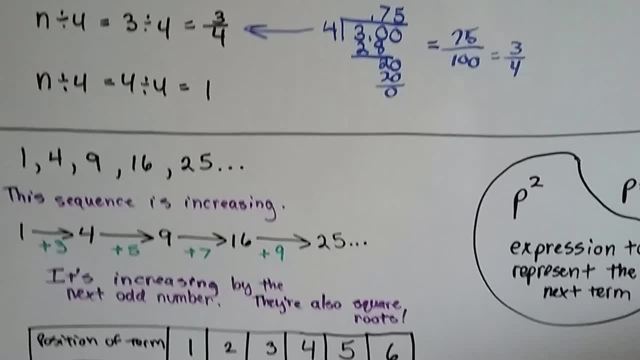 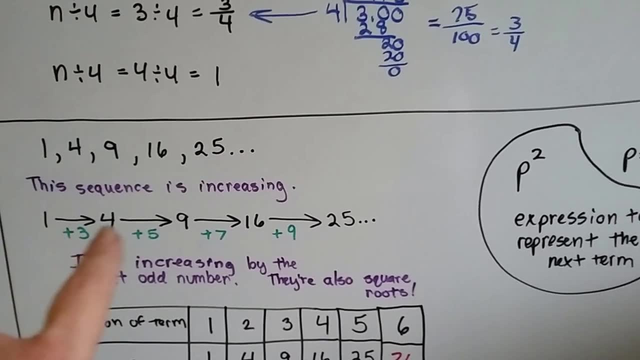 And 4 divided by 4 is 1, see What if we had this one: 1,, 4, 9,, 16,, 25.. Well, we can see the sequence is increasing, And then we can draw the addition in between them to see what's happening. 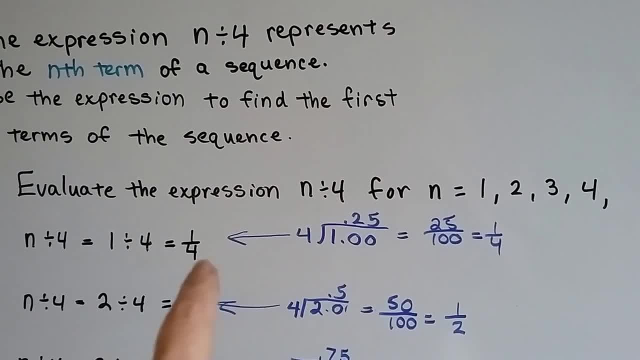 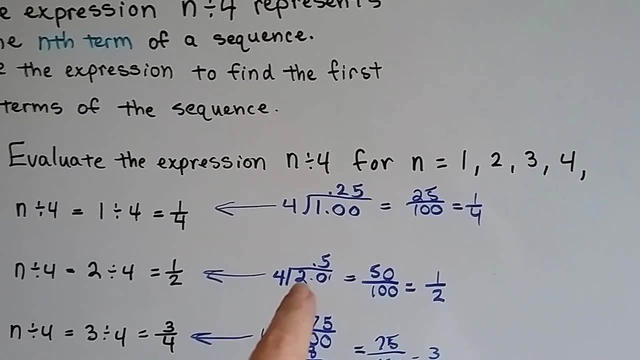 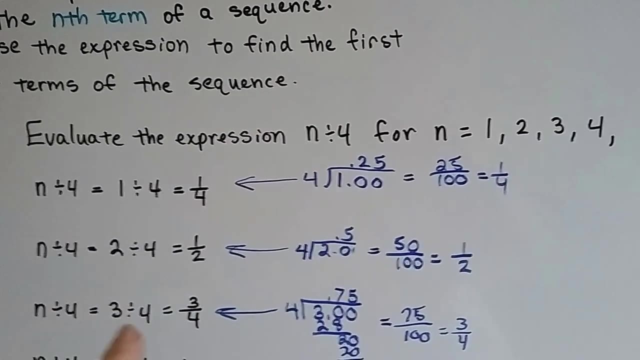 by 4 is 0.25 or 25 hundredths or 1 fourth. If n divided by 4,. if the n was a 2, see then it would be 2 divided by 4, which is 0.50 or 50 over 100 or a half. If it represented a 3, it would be 3.